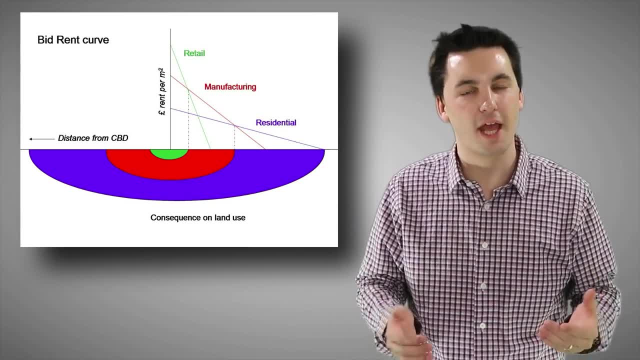 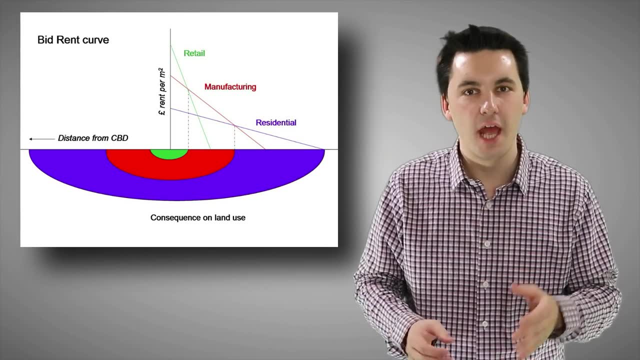 Our population density is lower, meaning demand for that land is less, So the price goes down. This is going to be important for us to understand when we're looking at the spatial layout of different cities, especially when we're trying to understand the location of different commercial, industrial and residential zones. 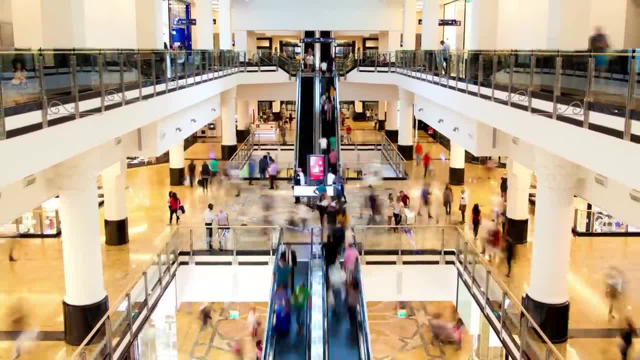 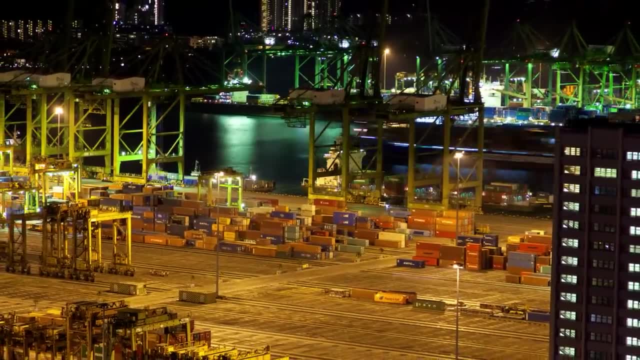 We can see that large retail stores and specialized services that make more money are more likely to locate near the central business district, or CBD for short, where industrial zones that require a lot of workers but do not need to be right next to that central business district are located farther out With 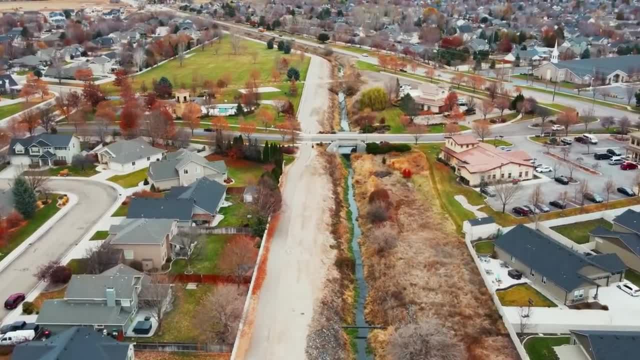 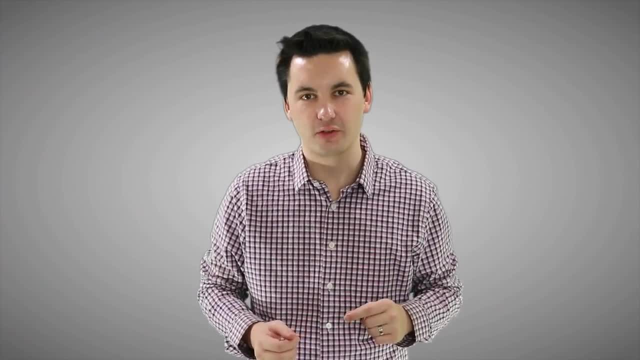 residential zones, often located after that. This is to minimize costs and to maximize their productivity. By understanding the bid-rent theory, we can see the spatial layout of our cities. Now, one thing that bid-rent theory doesn't do a good job of is predicting where people might live, based on income at least. And that's because sometimes people will rent. They'll rent a multi-family unit, They'll be renting an apartment or maybe even a condo, So the price of land isn't factored into it, since they're not purchasing it. Instead, they're renting from a landlord. So we've reviewed the bid-rent theory. Now we're going to move into Burgess' concentric zone model and this is going to be our first urban city model. It was developed in the 1920s, based off the city of Chicago. 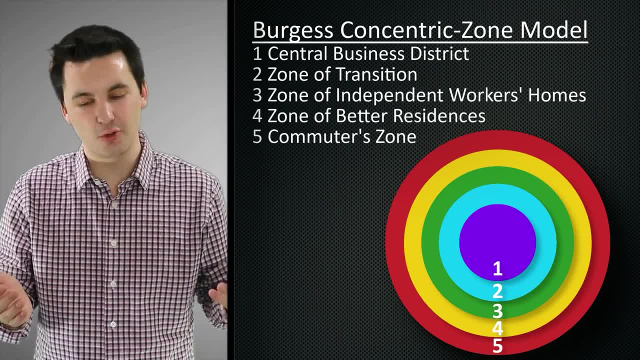 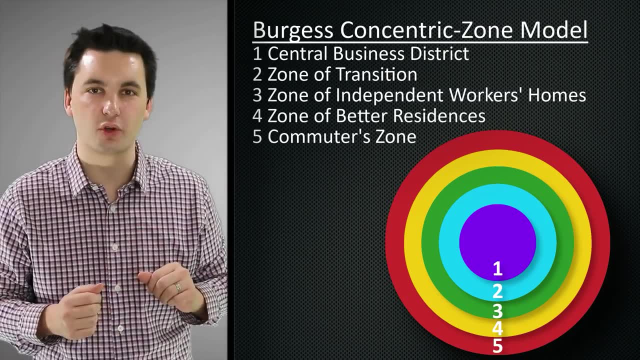 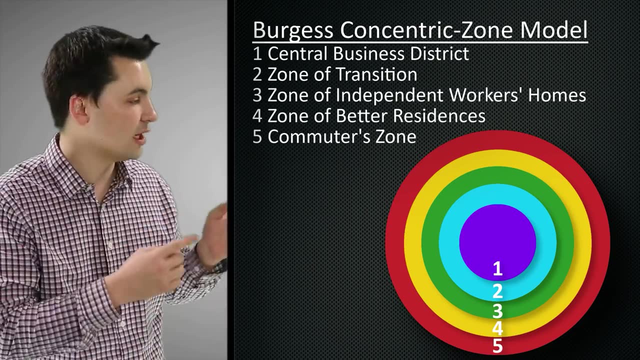 This model focuses on the different socioeconomic statuses of individuals and homes within a city. Traditionally, this model has older homes located closer to the central business district, with newer development happening further out. Lower-income residents and industries are often located in the zone of transition. 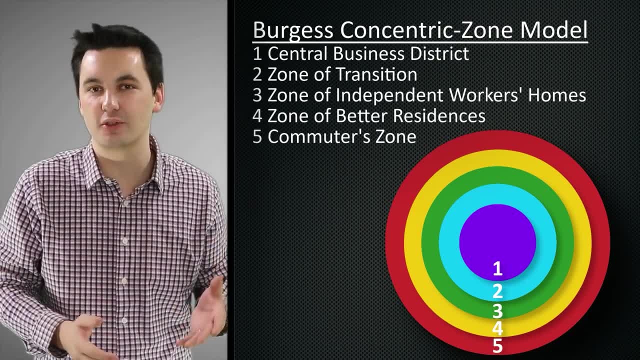 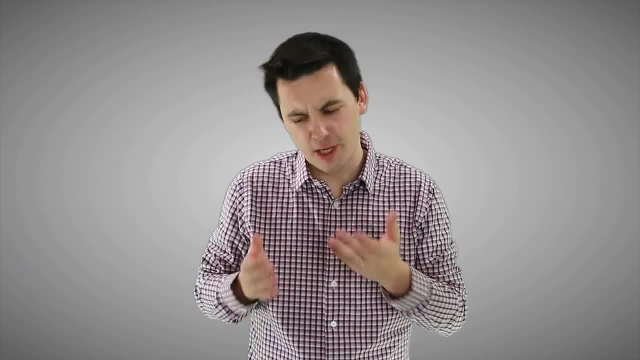 However, this is more for the United States. We can actually see in countries in Europe that more of the wealthy individuals are located closer to that CBD. Now parts of this model are starting to change and, quite frankly, it's becoming a little outdated. 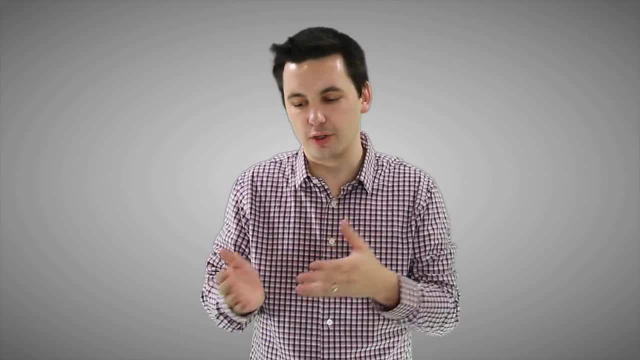 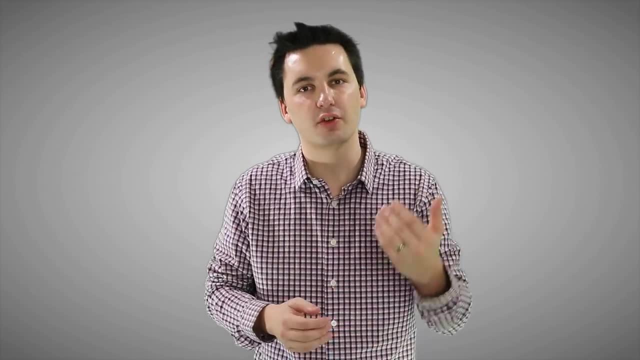 And that's due to globalization, changes in the production of our goods and services, gentrification and also urban renewal policies. All of this is starting to change where we're living, the price of homes and also the location of different industries. 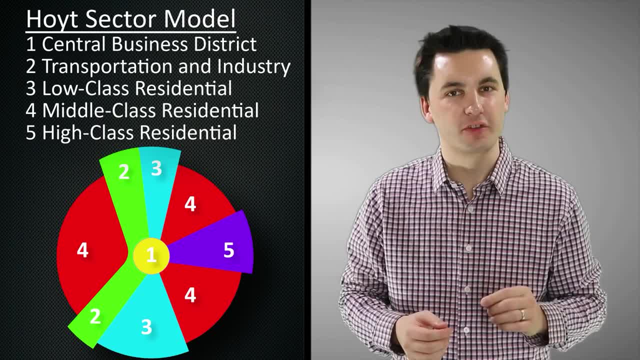 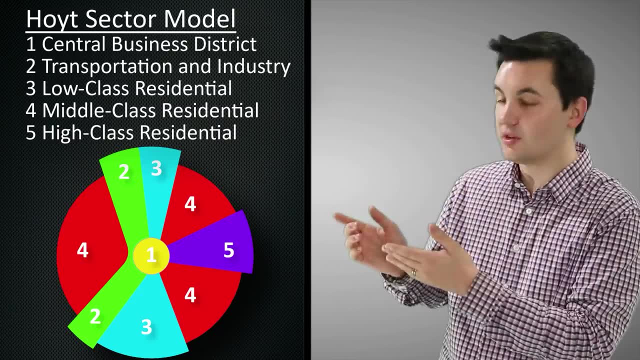 The next model is the Hoyt sector model, and this model still uses the CBD as the center point of the model. However, this model doesn't develop in a series of rings. Instead, we can see it develops in a series of wedges or sectors. 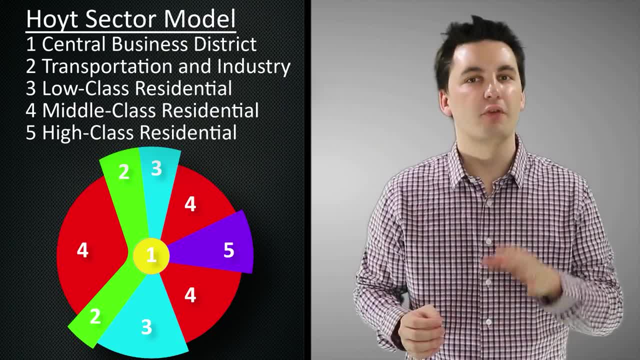 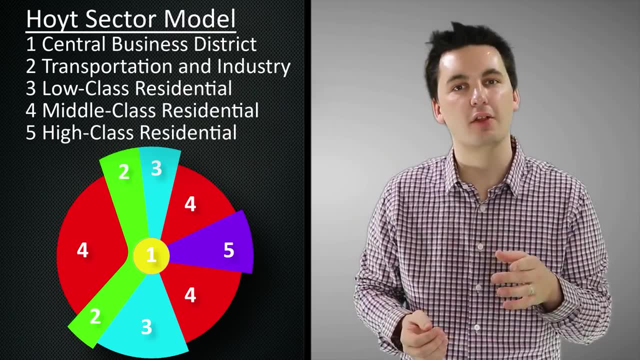 This is based off different economic and also environmental factors. For example, industries we can see will actually align near transportation systems, highways and railroads. This will allow them to be able to export their goods quicker and also be able to connect with their consumers. 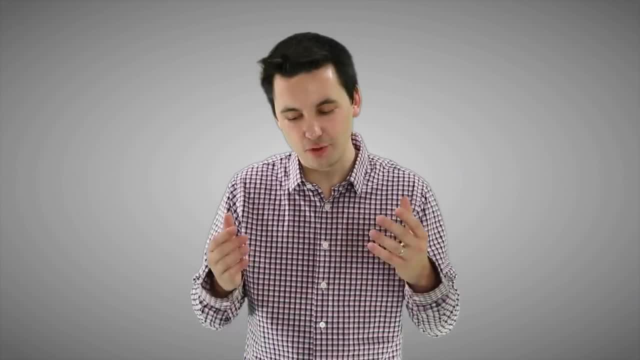 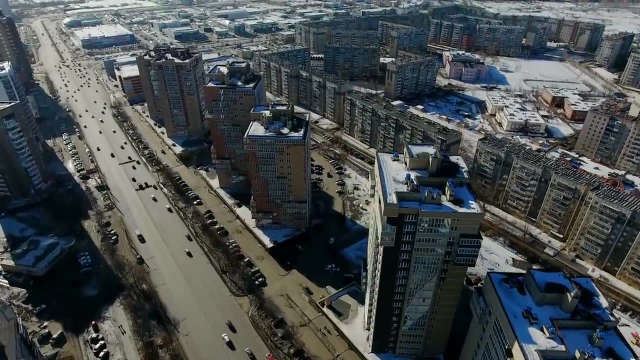 Now, just like our previous model, this model is also experiencing changes and it's starting to feel a little dated, And that's because of changes in our transportation system, Also infrastructure. People are living now farther away from cities, which means businesses are moving with them. 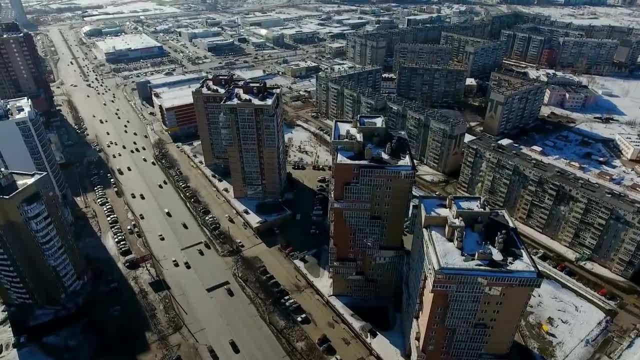 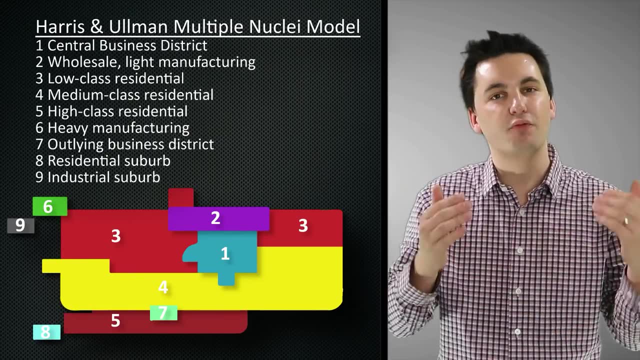 So we're seeing some changes in the location of different people and also businesses. The next model we have is the Harrison-Ullman multinuclear model. This model was created around 1945, and it focuses on trying to account for the changes in technology and also transportation that society was seeing. 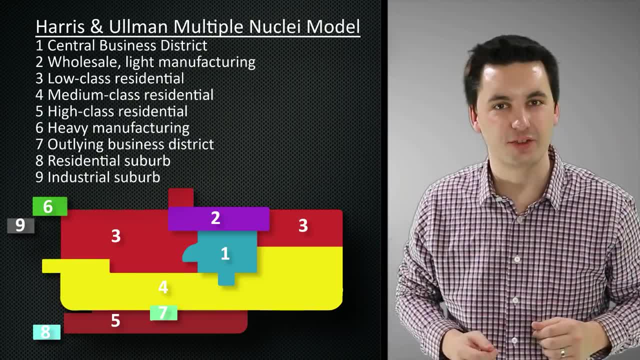 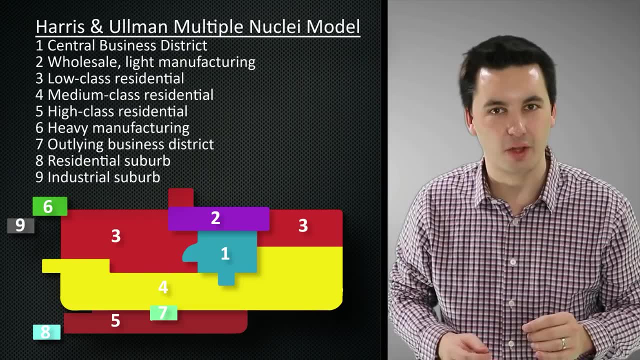 We can see when looking at the model that it has multiple central business districts. Now we still have our original CBD, But this city now has multiple CBDs, each around their own purpose. We can see that the CBDs will have unique economic opportunities for residents in that city. And these CBDs will act as nodes within the city. They'll attract certain industries, people and organizations based on what's offered in those CBDs. Hence why we have multiple central business districts. They all serve different purposes. For example, CBDs are nodes of the city that focus on manufacturing and are more likely to see the workers of those factories. 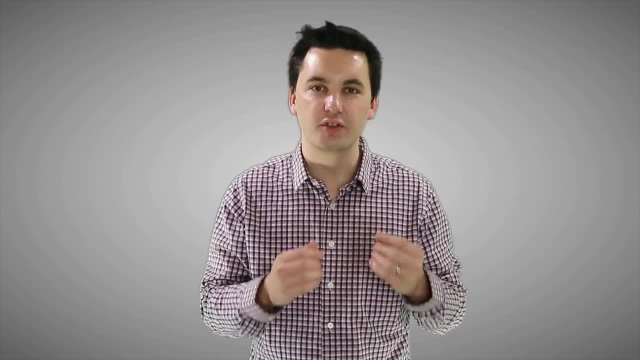 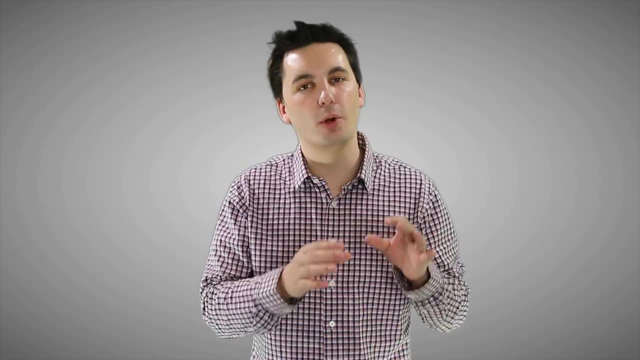 within that area. On the other hand, though, we could also see certain CBDs of the city or nodes repel others. For example, again if we go back to our manufacturing part of the city, it's more likely that the more wealthy individuals of a community aren't going to want to live near that CBD. 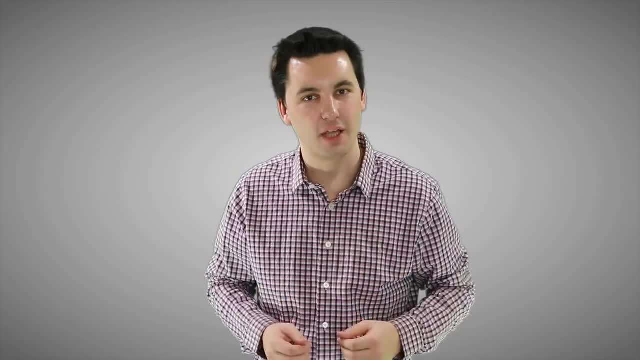 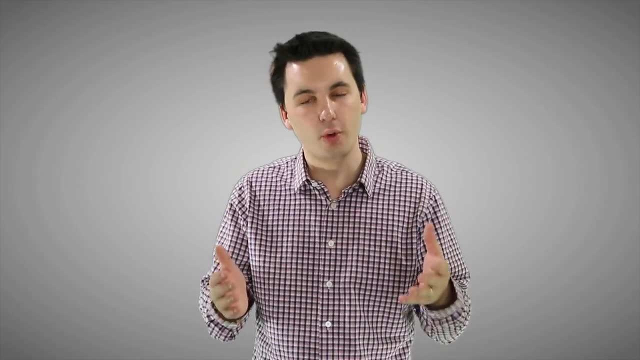 And they're more likely to live by a CBD that focuses on their way of life. So we can see that the city actually can become kind of segregated. That could be kind of an issue based on economics, but also based on the opportunities provided throughout the different cities. 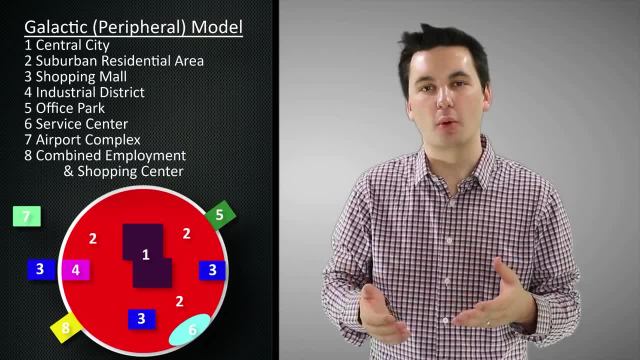 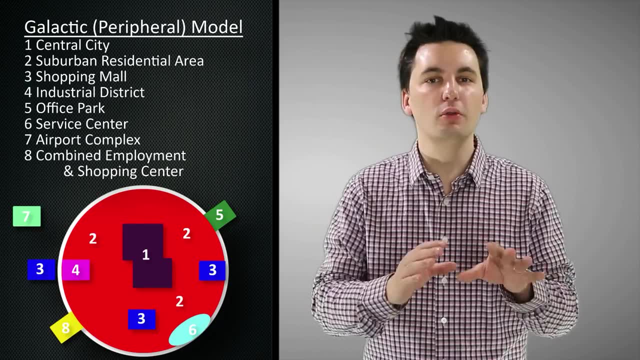 Continuing off of our multinuclear model, we can go into the next model, which is our galactic model. This was made around the 1960s and it tried to address the changes in the economy. No longer are we seeing cities that are focused on manufacturing. 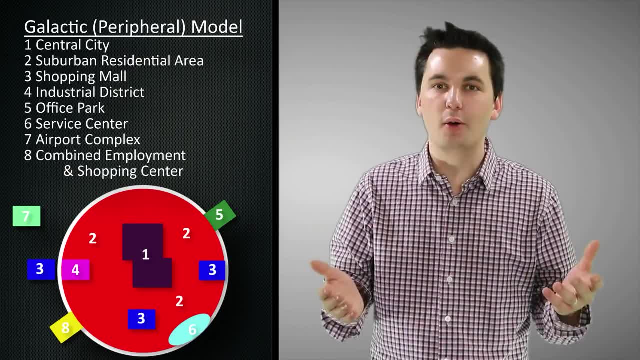 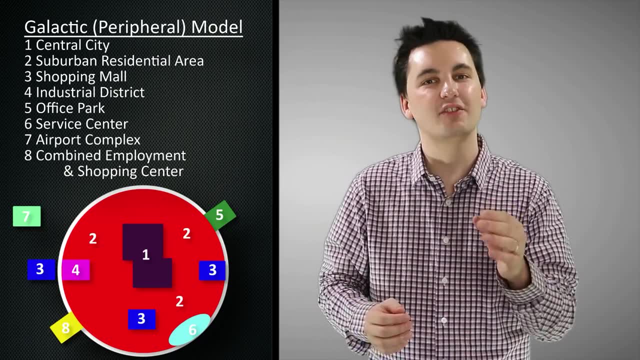 Now we're past. post-industrialization Cities now are focusing on more services And thanks to advancements in transportation and also our new robust infrastructure systems, we can see that people are now living farther away from that central business district. This model has edge cities. 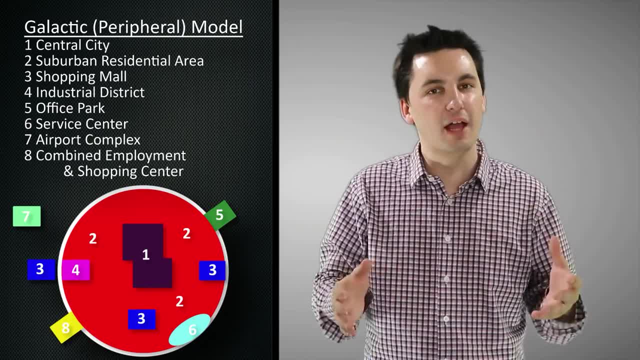 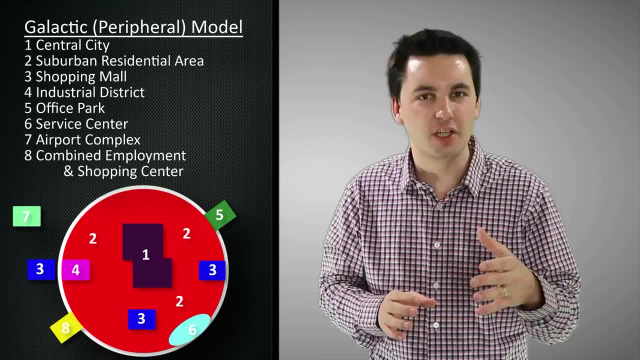 Which we can see are connected by a beltway or a highway. This allows these edge cities to offer more specialized services, as they're connected to other edge cities. If you need more information on the edge cities, the beltways, check out my video on 6.2.. 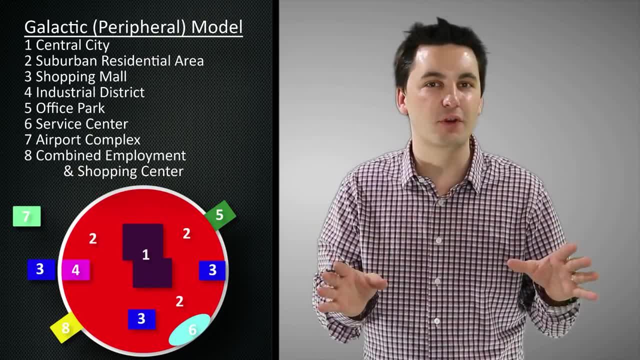 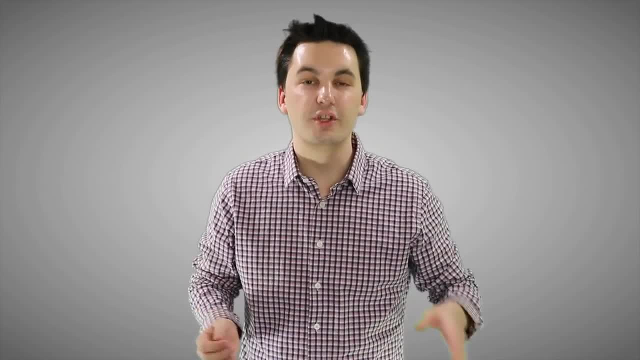 It goes into edge cities, boom burbs, X burbs and all these different concepts that apply to this specific model. Now, so far, we've been talking about city models that focus on the United States and North America. The next three city models we go into, though, are going to focus on different regions around the world. With the first being the Latin America, The Latin American city model. This model takes aspects of the concentric zone model and also our sector model, And we can see the influence of colonization on this model as well. Here, the CBD is still located in the center of the model. 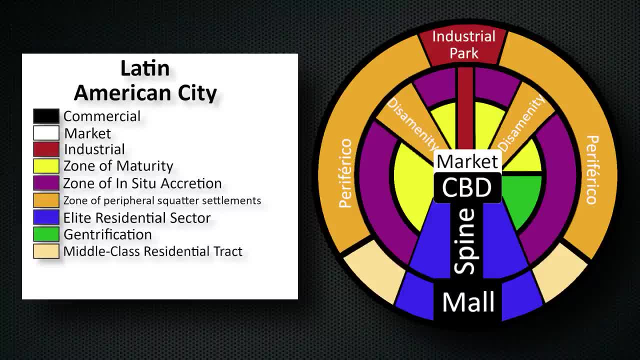 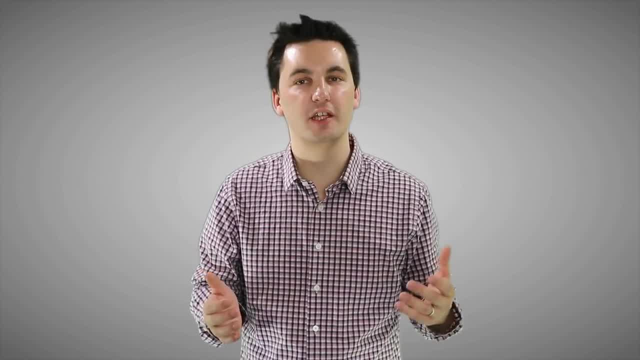 With a spine which goes to the mall, And the spine has most of the high wealth residents. In this model we can see the division between different socioeconomic classes, With some parts of the city living in extreme poverty. This is known as the disamenity zone. 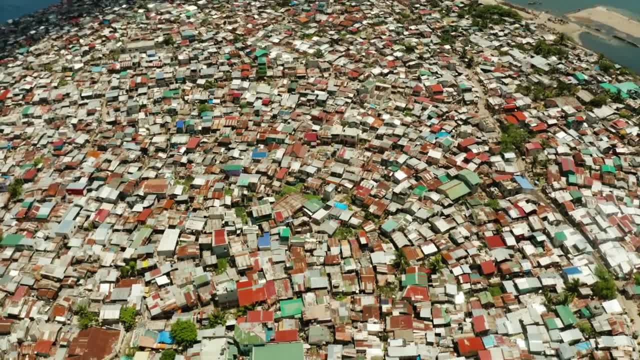 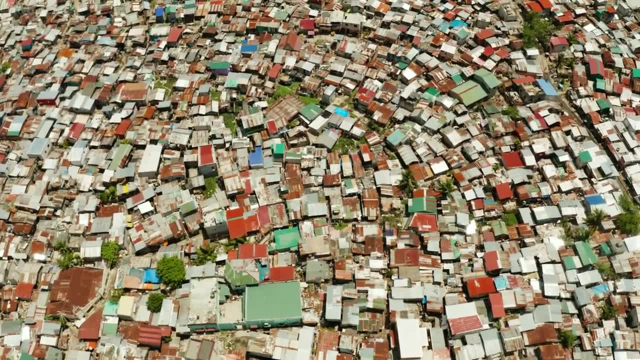 In some cases and in some parts of the city, unfortunately, we'll see areas that lack basic infrastructure- Things like water, power and sewage- And also, in this model, we'll see squatter settlements starting to form. These traditionally, are happening on the outside of the model. 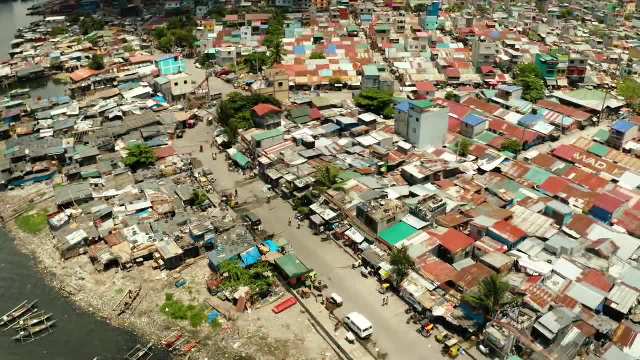 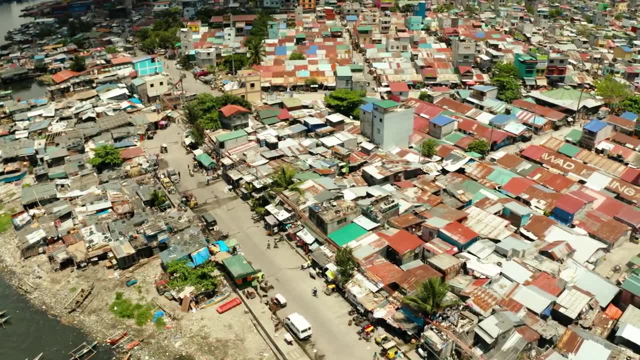 And it's due to this increased urbanization that's happening. As these countries develop, we're starting to see more people be drawn into the city. Unfortunately, that's putting further pressure on these urban areas And they're not able to provide services for all of the people. 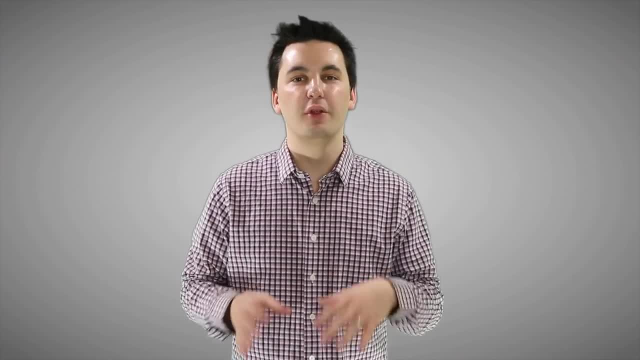 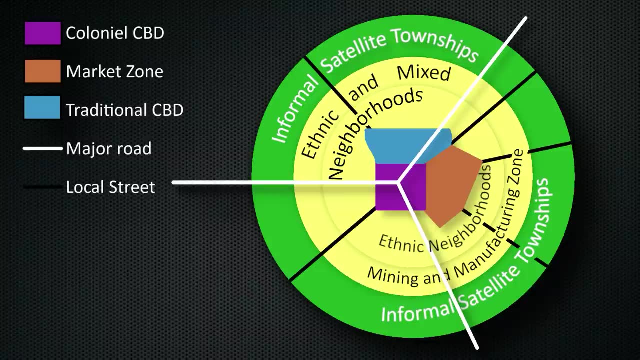 If we move over to Africa, we can see the sub-Saharan African city model. These models have a significant amount of influence from their European colonizers. These cities often have three CBDs: A traditional CBD, A CBD built by European colonizers, with more of a grid-like pattern in their streets. 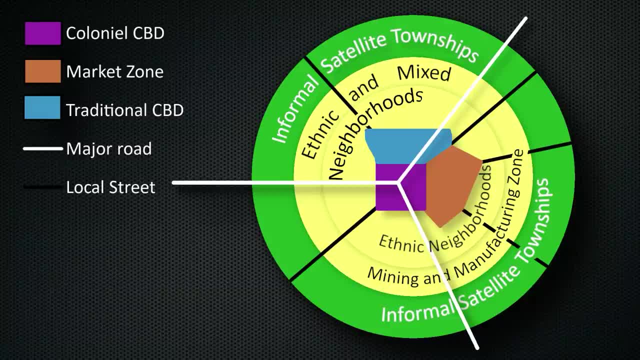 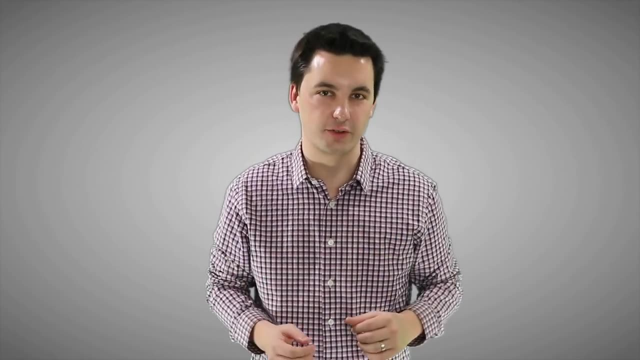 And multi-story buildings resembling the architecture of European countries And, lastly, an open market. CBD Infrastructure in these cities is more robust near the city center, Similar to the Latin American city model. we start to see shanty towns and squatter settlements form on the outskirts of the city. 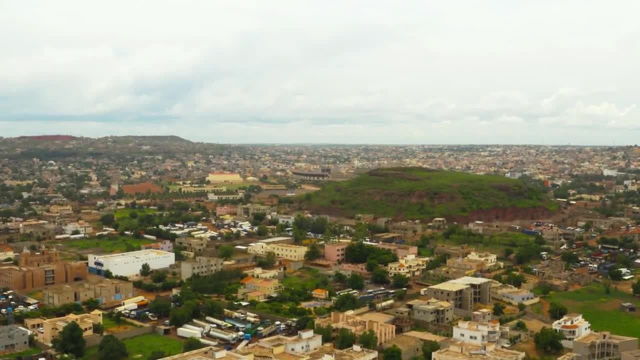 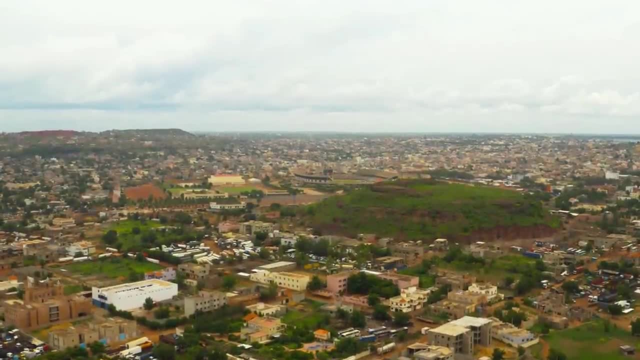 This is because, as countries continue to develop and advance in the demographic transition model, we start to see more urbanization As more job opportunities focus in these larger cities, we see people migrate from rural areas into urban centers. Lastly, we could also look at the Southeast Asian city model.